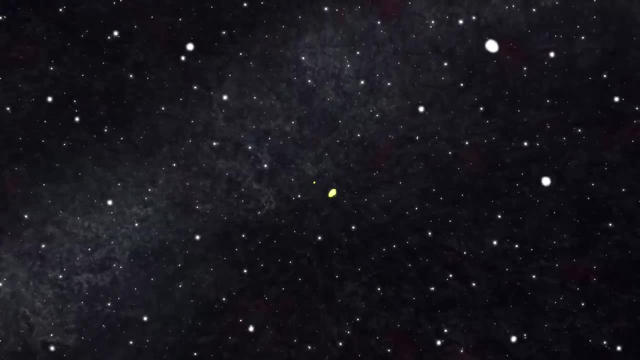 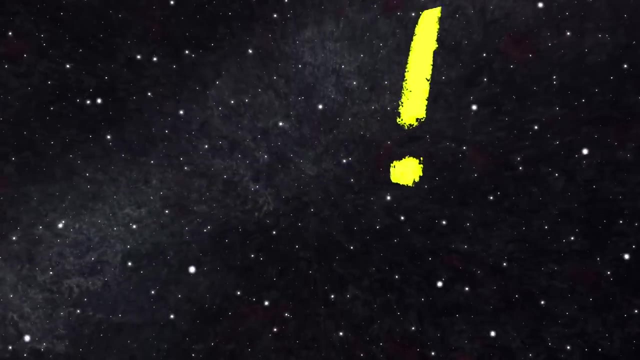 and our place within it. some of the unknowns get better known and we can estimate an answer a bit better. But there won't be a definite answer to the Drake Equation until SETI succeeds or something else proves that earthlings are the only answer. 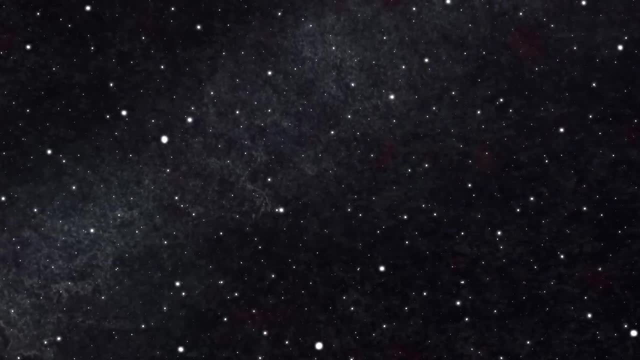 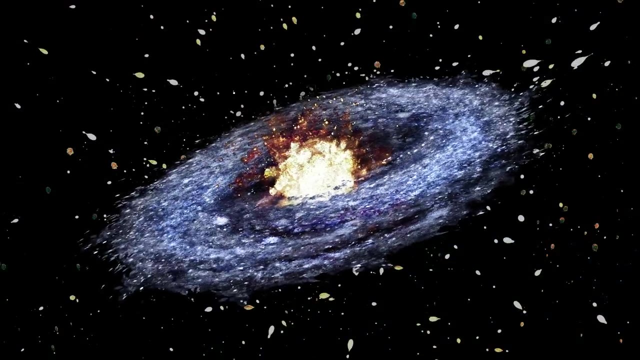 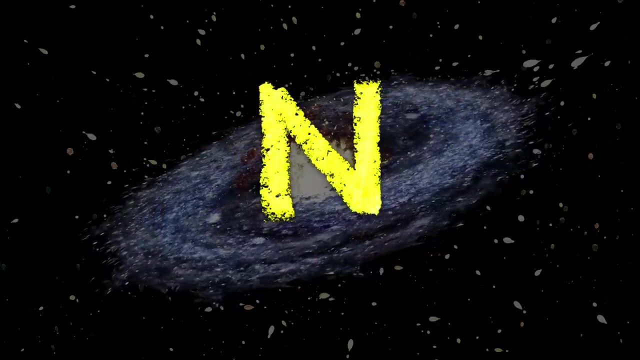 In the meantime, it is really useful to consider the unknowns. The Drake Equation attempts to estimate the number of technological civilizations in the Milky Way galaxy with whom we could make contact, and it's usually written as: n equals r star multiplied by f, sub p multiplied. 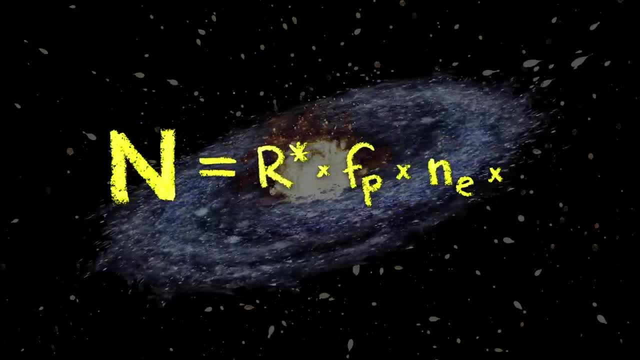 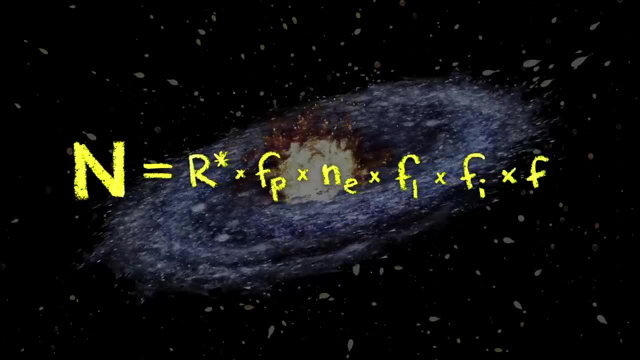 by n sub p, So h sub i, multiplied by n sub p, multiplied by n sub p, multiplied by n sub e, multiplied by f sub L, multiplied by f sub i, multiplied by f sub c and, lastly, multiplied by capital. 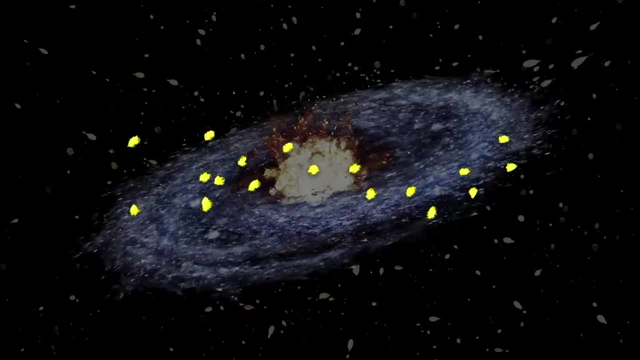 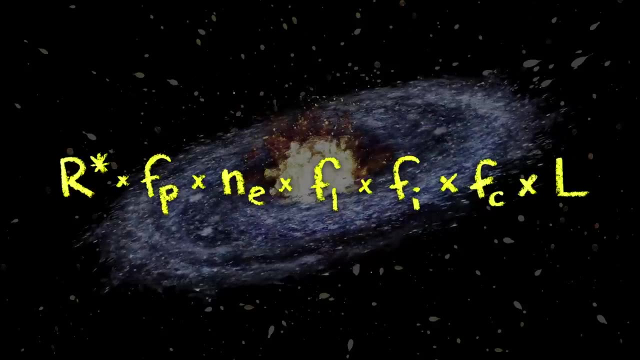 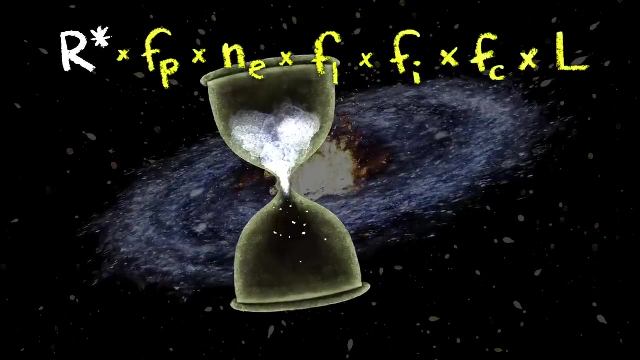 L. All those factors multiplied together help to estimate the number of technological civilizations that we might be able to detect right now. Our star is the rate at which stars have been born in the Milky Way galaxy- born in the Milky Way galaxy over the last few billion years. so it's a number. 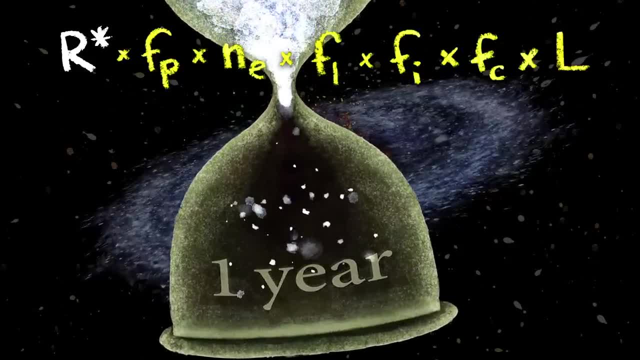 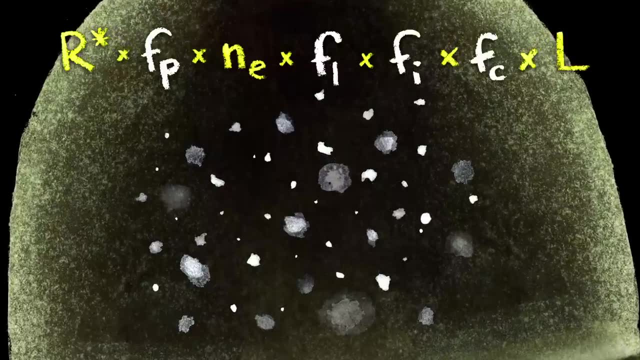 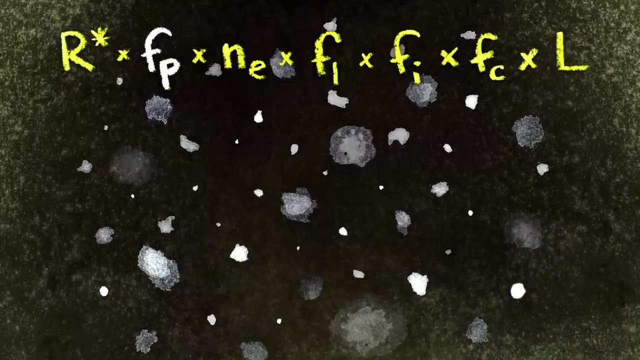 that is, stars per year. Our galaxy is 10 billion years old and early in its history stars formed at a different rate. All of the F factors are fractions. Each one must be less than or equal to one. F sub P is the fraction of stars that have 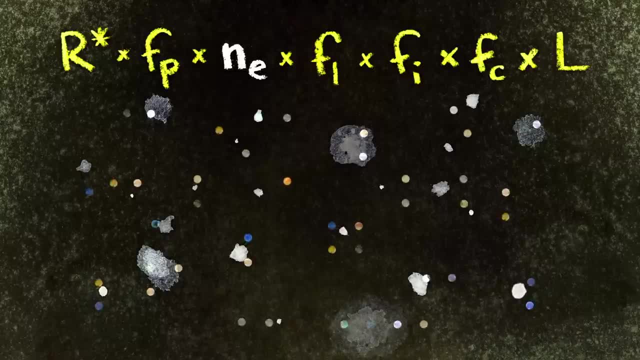 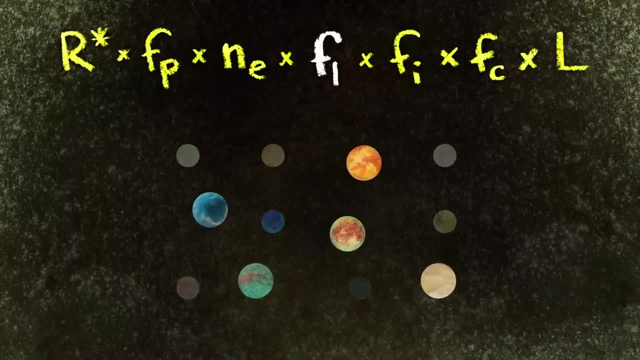 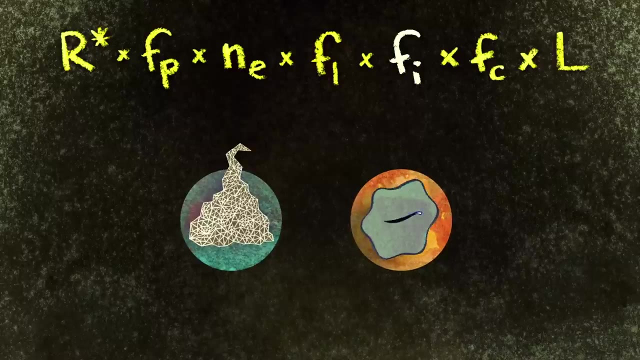 planets. N sub E is the average number of habitable planets in any planetary system. F sub L is the fraction of planets on which life actually begins, and F sub I is the fraction of all those life forms that develop intelligence. F sub C is the fraction of intelligent life that develops a civilization that 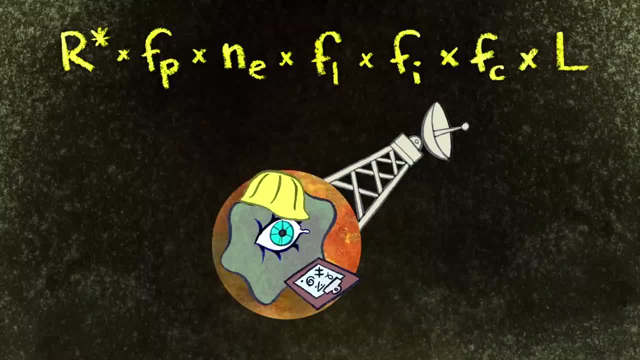 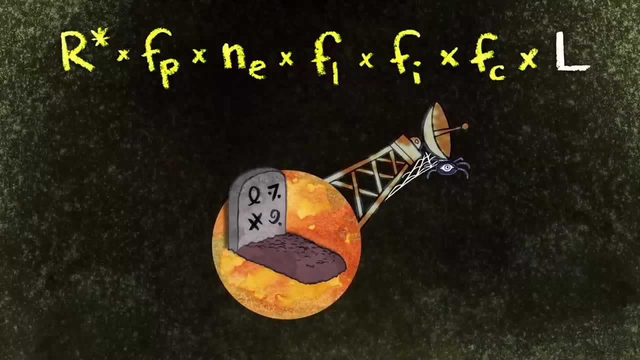 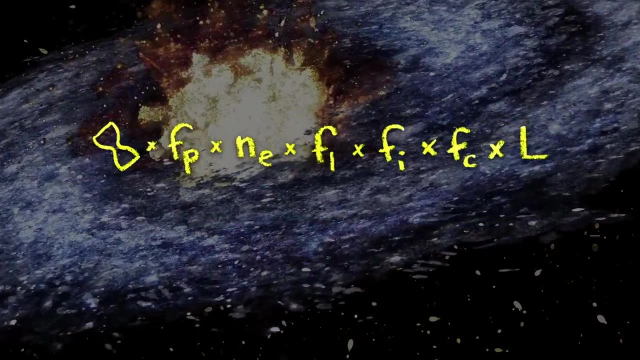 decides to use some sort of transmitting technology. And finally, L, the longevity factor. On average, how many years do those transmitters continue to operate? A star is the average number of lives that a planet has. Astronomers are now almost able to tell us what the product of the first three terms is. 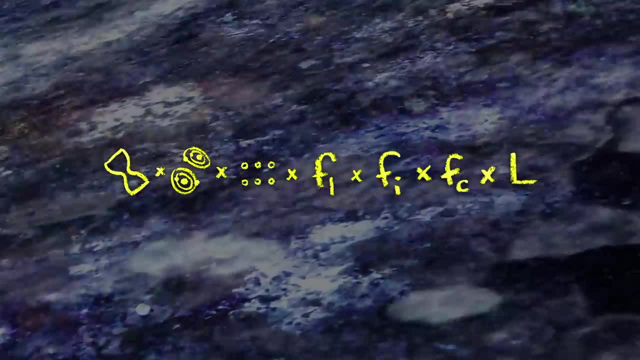 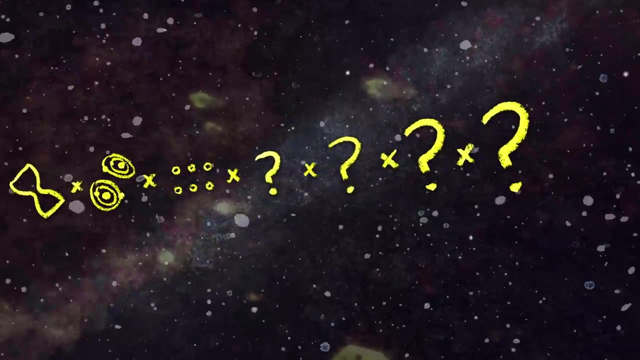 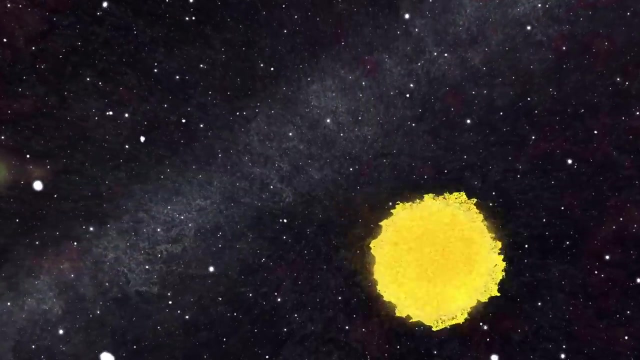 We're now finding exoplanets almost everywhere. The fractions dealing with life and intelligence and technological civilizations are ones that many, many experts ponder, but nobody knows for sure. So far, we only know of one place in the universe where life exists, and that's right here on Earth. 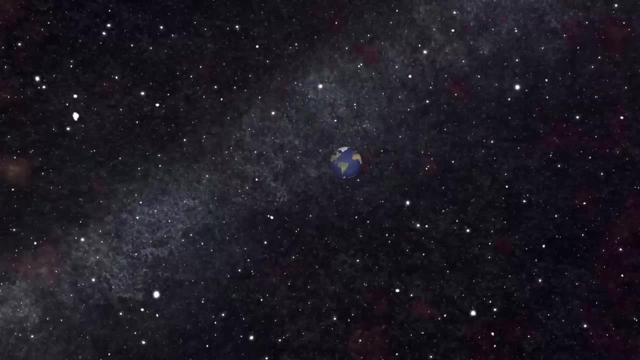 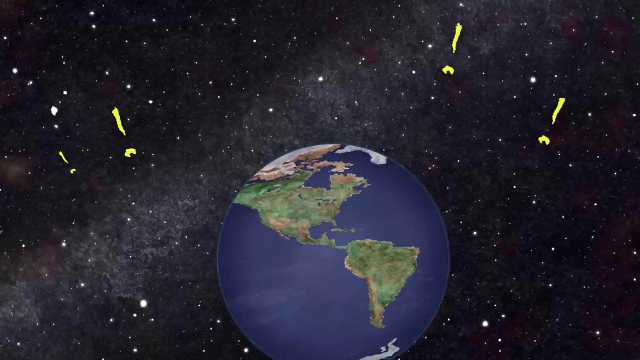 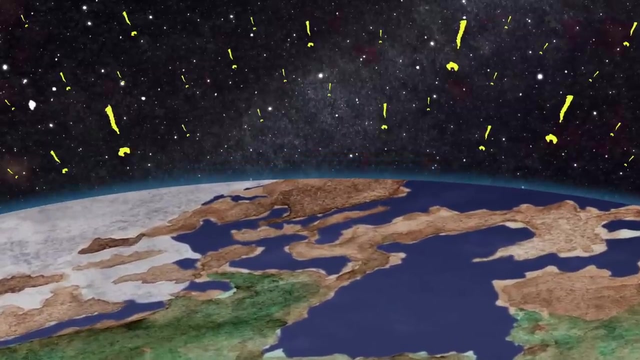 couple of decades as we explore Mars and Europa and Titan. the discovery of any kind of life there will mean that life will be abundant in the Milky Way, Because if life originated twice within this one solar system, it means it was easy And given similar conditions elsewhere. 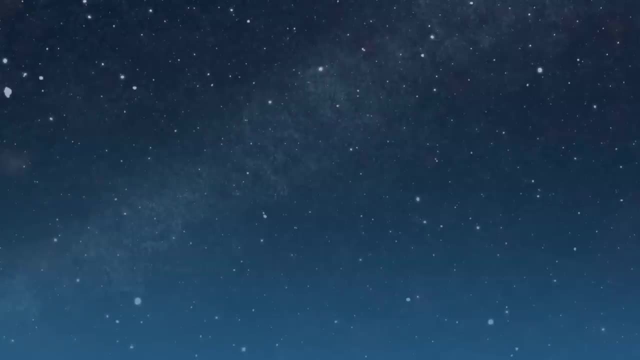 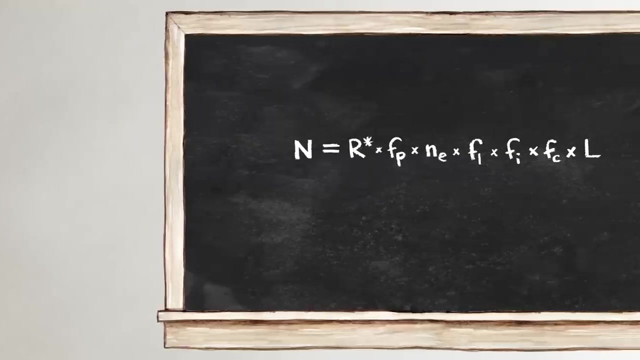 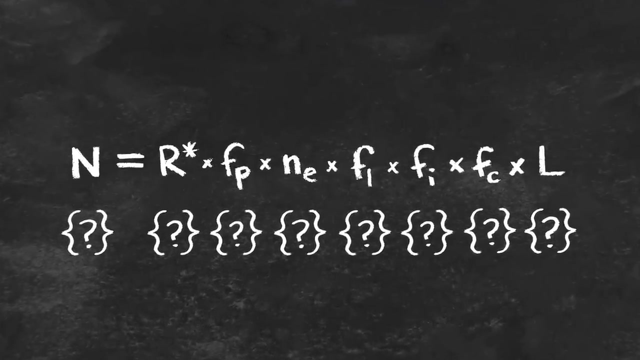 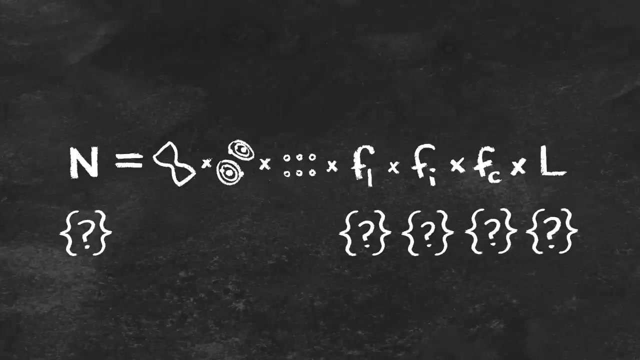 life will happen. So the number two is a very important number here. Scientists, including SETI researchers, often tend to make very crude estimates and acknowledge that there are very large uncertainties in these estimates in order to make progress. We think we know that r star and n sub e are both numbers that are closer to 10 than, say, to 1.. 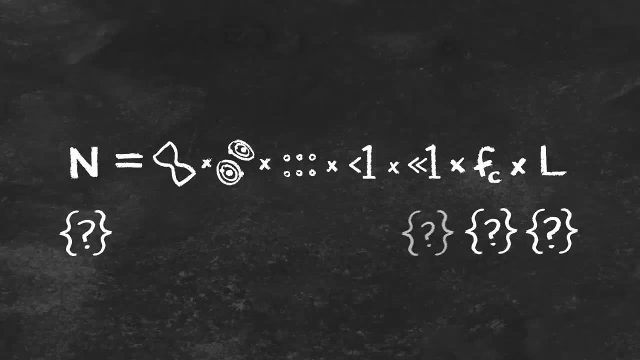 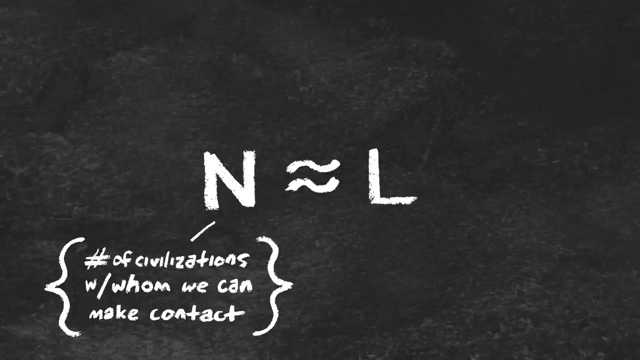 And all the f factors are less than 1.. Some of them may be much less than 1. But of all these unknowns, the biggest unknown is f. So perhaps the most useful version of the Drake equation is simply to say that n is approximately. 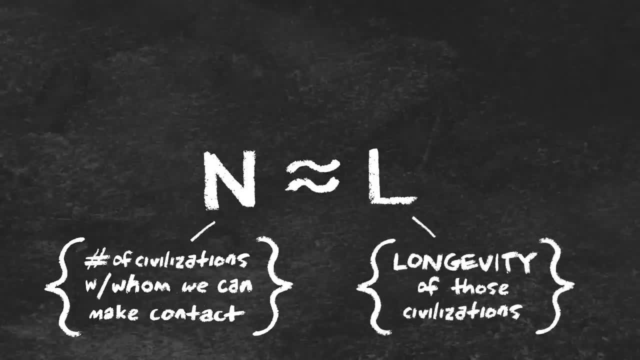 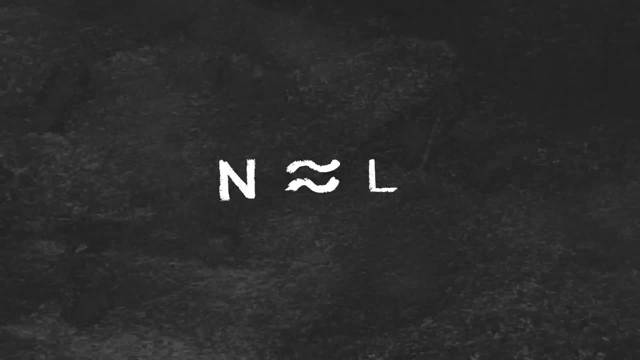 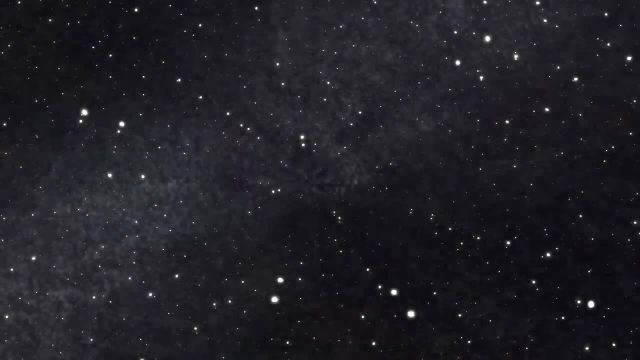 equal to l. The information in this equation is very clear. Unless l is large, n will be small. But you know you can also turn that around. If SETI succeeds in detecting a signal in the near future, after examining only a small portion of the star system, it will be very clear that n is 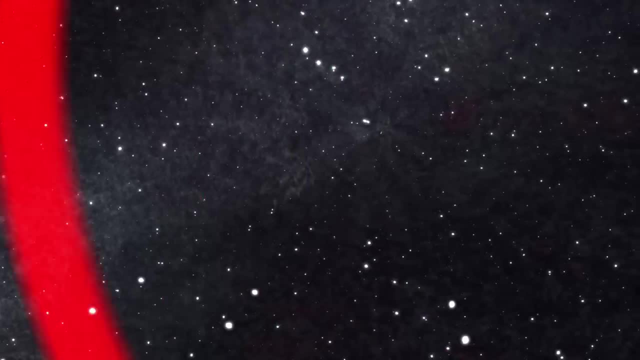 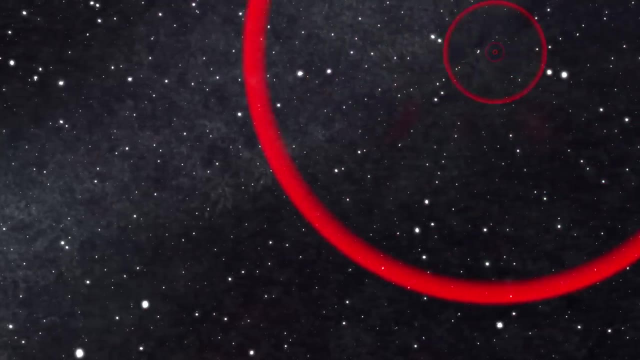 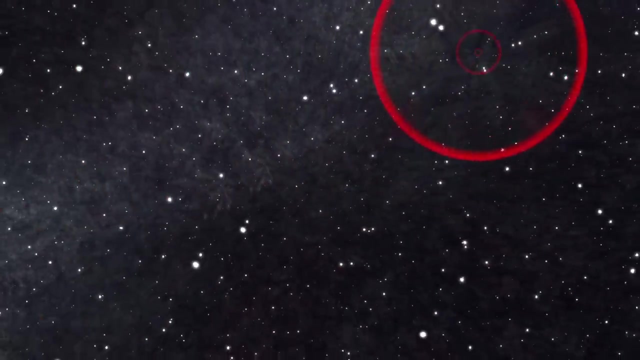 in the Milky Way, Then we learn that l on average must be large, Otherwise we couldn't have succeeded so easily. A physicist named Philip Morrison summarized this by saying that SETI is the archaeology of the future. By this he meant that, because the speed of light is finite, any